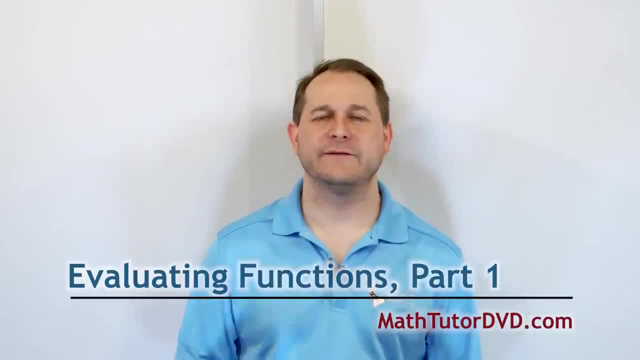 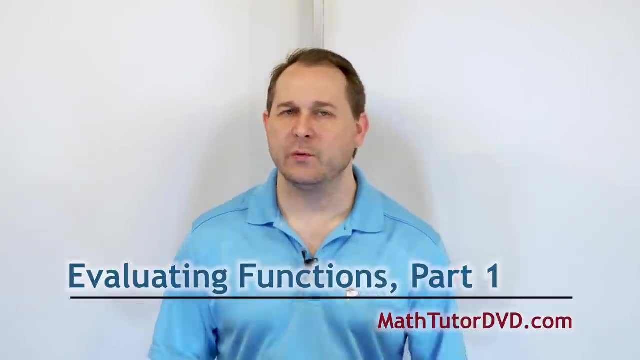 Hello, Welcome back to Algebra. The title of this lesson is called Evaluating Functions, Part 1.. In the last lesson we talked about the concept of a function. in algebra, which you'll be using functions pretty much forever, so just kind of get used to the idea. But 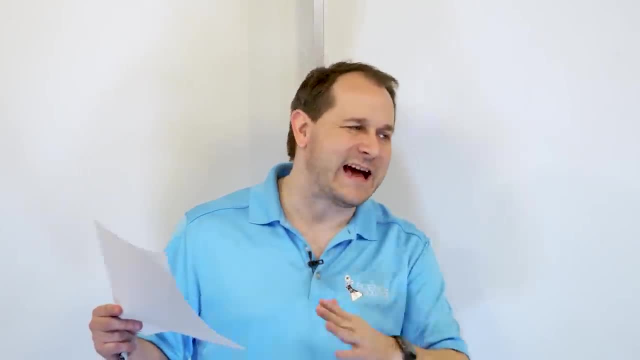 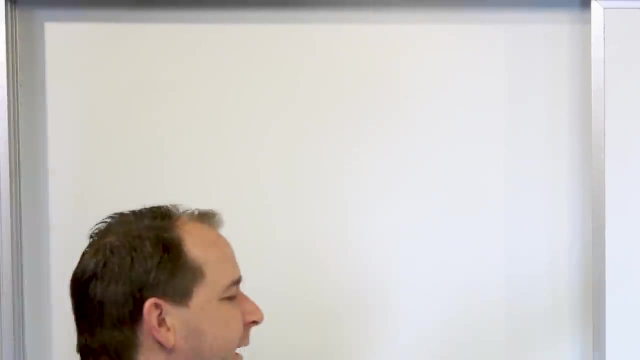 it's a machine that takes input values in x and then it calculates and it gives you the output values that we call f of x. So this lesson is all about doing those practice calculations, and we call it, by the way, evaluating the function is what we call it when we take 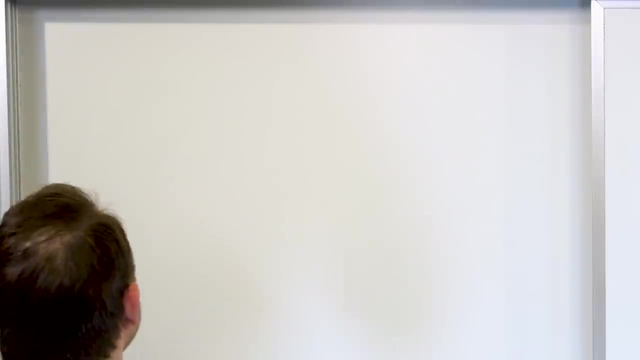 that input and we calculate the output. We call it evaluating the function. So if you had a function, f of x is equal to a very simple function, x plus 2.. First of all, what kind of function is this? You should recognize this as a line: mx plus b, so you know it's. 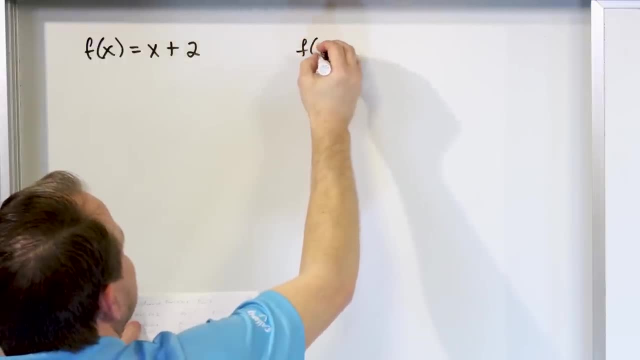 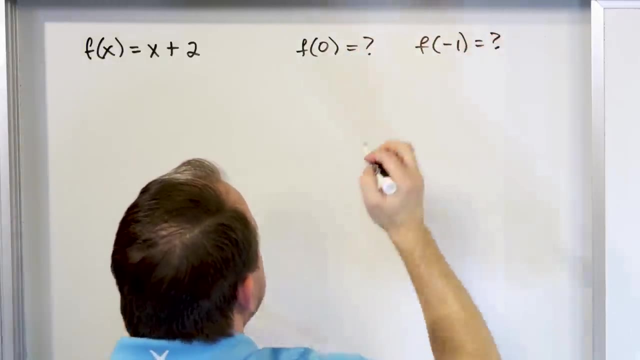 a line And we say we want to evaluate the function at x is equal to 0 and evaluate the function at x is equal to negative 1.. So when the value that we put in the middle here, this tells me the value of x that I want to evaluate the function at and I want to do 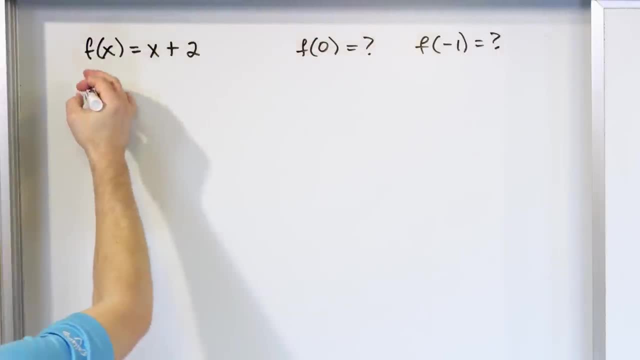 it two different times. So the way you write it mathematically is: you write the f, you open the parentheses and you take the value that you're trying to evaluate and then you substitute it in for x. So 0 plus 2, as you all know, is 2.. So in your paper you just say: 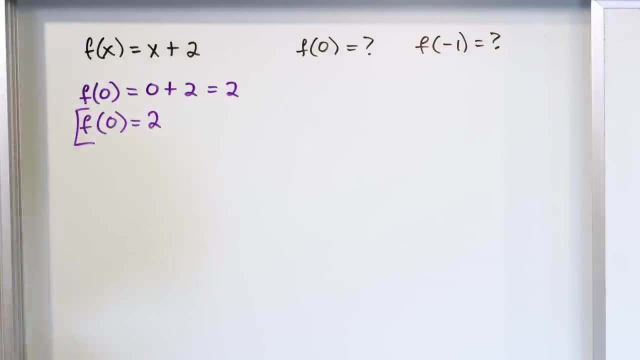 f of 0 is equal to 2.. This is what you write down. Now you have to be careful, because up until now we've been using parentheses to mean multiplication. But in this case, when we're writing functions down, It never means multiplication. It means the function f, evaluated at x, is equal to 0, gives the value 2.. 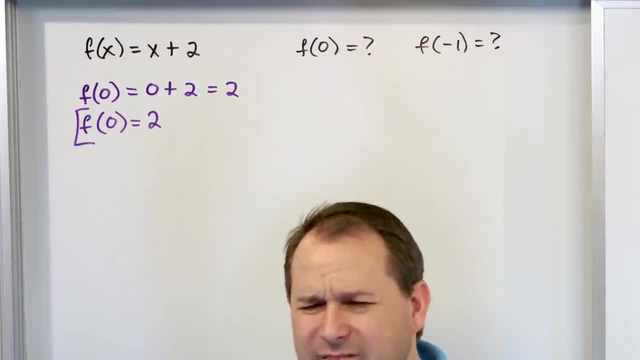 That's what this means. So it does not mean f times 0.. And, by the way, the letter f is almost never used for anything in math other than functions. So when you see f, you always know it's a function. Now to do the other one. here we do exactly the same thing. 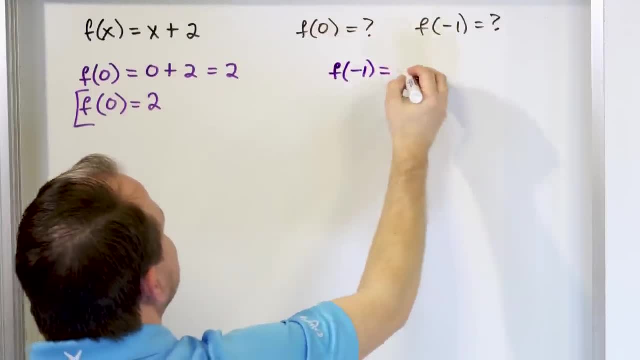 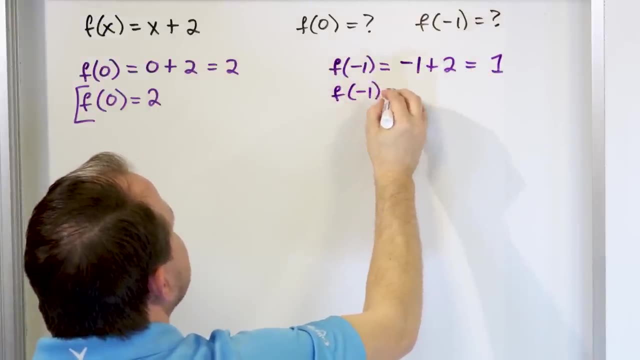 f evaluated at x is equal to negative. 1 means we stick negative 1 in here and we get. what do we get? 1.. Negative 1 plus 2 gives us positive 1. So we say: f evaluated at negative, 1 gives us 1.. 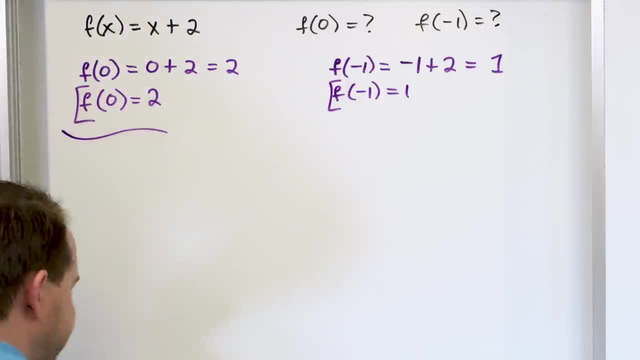 We circle those answers, So we're just going to continue working down the way here. This is mostly an exercise in substitution, but we're kind of getting used to the idea of what a function is. You also very commonly will see the function g to represent the letter g to represent a function. 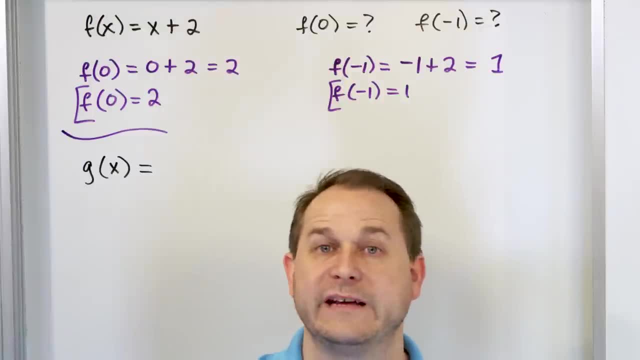 Basically, it doesn't matter what letter of the alphabet you use, but typically you'll see f, You'll see g in physics, Sometimes you'll see u and v, but almost always in algebra it's going to be f almost always. sometimes g of x. 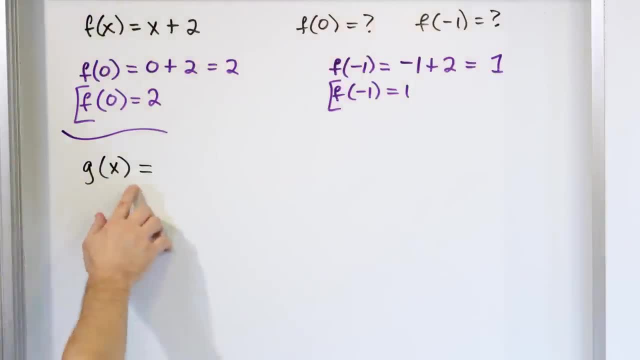 So just kind of get used to that. You might see g of x representing a function that we're naming g. So this function of x is 1 minus 2 times whatever x is, And let's say we want to evaluate it at x is equal to negative 2 and we want to evaluate it at x is equal to positive 3.. 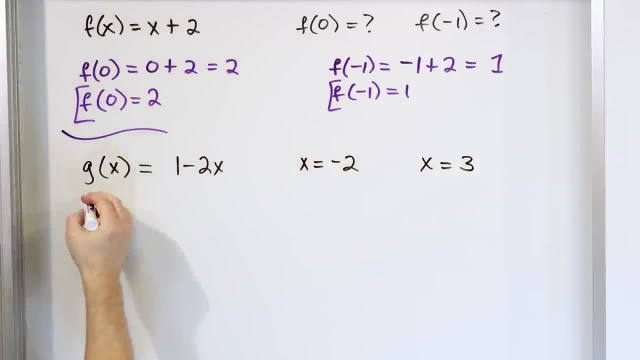 So how do we evaluate that? We take these values in and we stick them into the function. g evaluated at negative 2 means that we take and then we stick it right into the value of x here, So we have 1, then we have a minus sign here, but this multiplication is actually negative 4.. 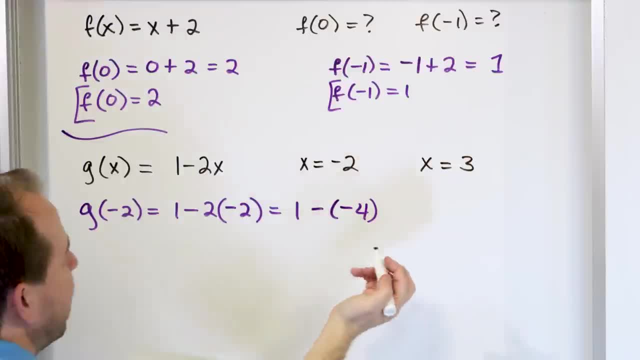 Minus, and this multiplication is negative 4.. Or you could write it as 1 plus 4,. however you want to do it, It's going to end up being 1 plus 4.. And so you're going to end up with 5 for the answer there. 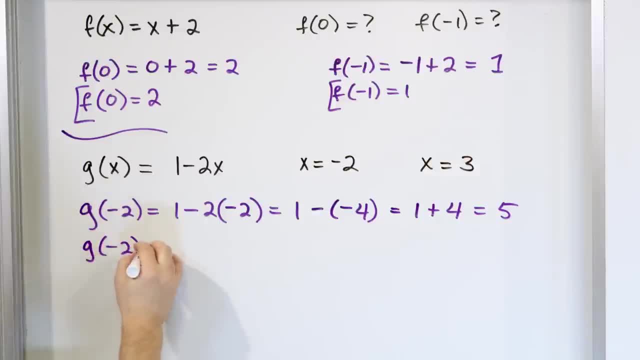 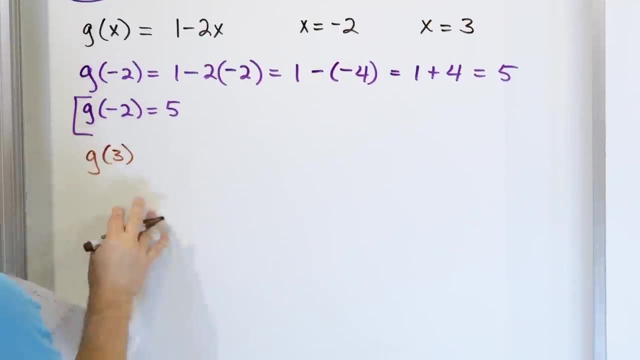 And so what you're going to get is g evaluated at negative 2 is equal to 5.. And this is what you want to circle on your test. The function g evaluated at x is equal to negative 2 gives you this value. All right. so the next one, when x is equal to 3, means we take g, we evaluate it at the position of x equal to 3.. 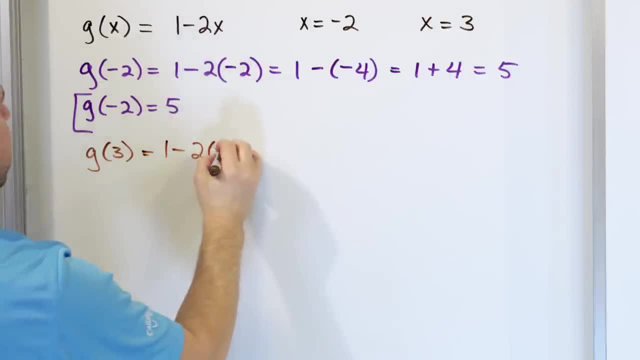 And we say it's 1 minus 2 times 3 in here. So it's 1 minus 6, and 1 minus 6,, as you know, is negative 5.. So g, evaluated at x, is equal to 3, is negative 5.. 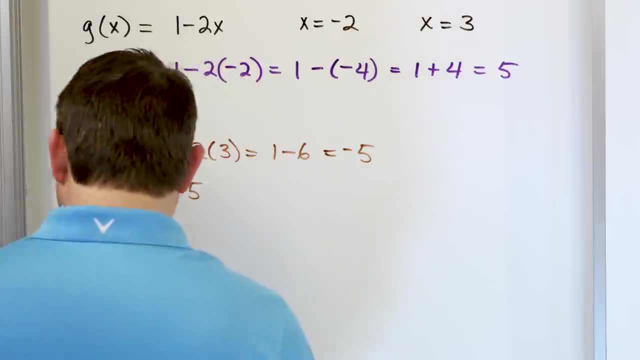 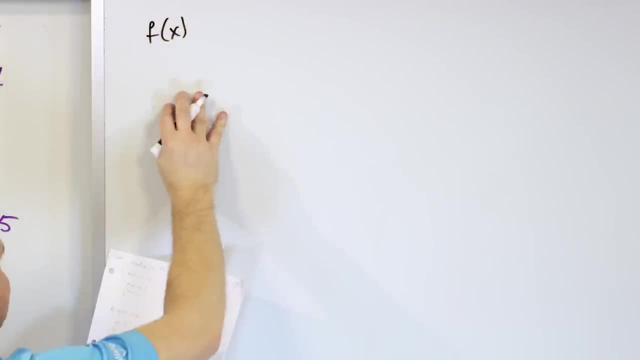 And that's the final answer for that one And again, we're just going to continue cruising along and doing different functions, getting slightly more complex each time. Let's say we have the function of x as being the absolute value of 2 minus x. 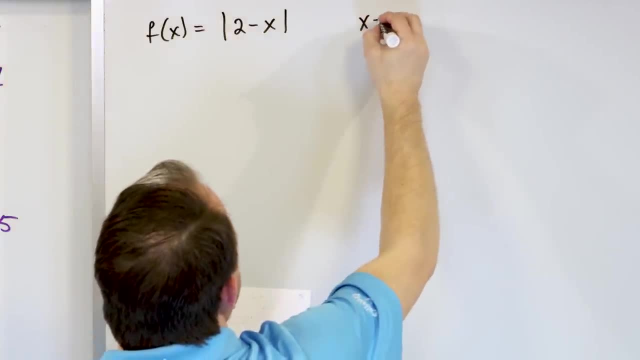 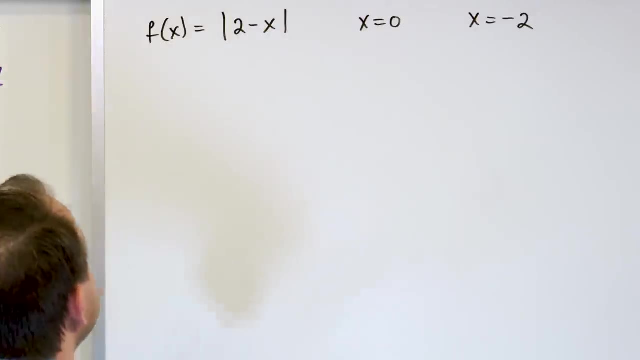 So now we have an absolute value in the mix and want to evaluate it when x is equal to 0 and also when x is equal to negative 2.. So we'll switch colors a little bit here and we will say f evaluated when x is equal to 0. 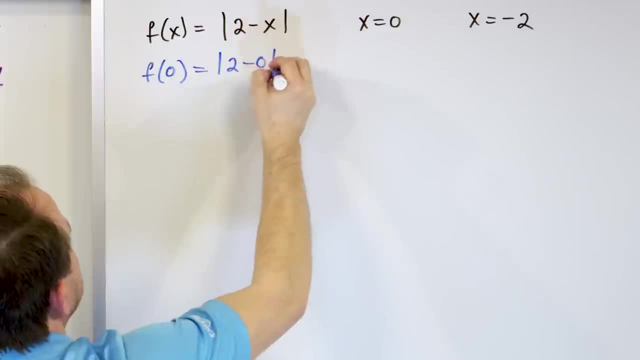 is equal to negative 2.. So f evaluated at x is equal to 2 minus 0, with the absolute value around it. So it means it's the absolute value of 2, which, as you know, is just 2.. So f evaluated at 0 is 2.. 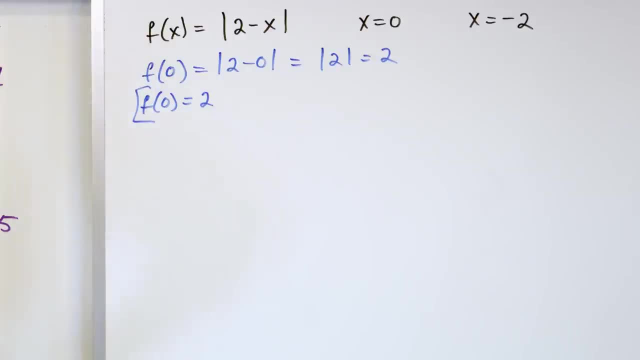 That's the function evaluated there as well. And then, finally, we will take the last one and we will say: f evaluated at x is negative, 2 is absolute value of 2 minus. now, be careful: it's minus, but x is negative, so you should. 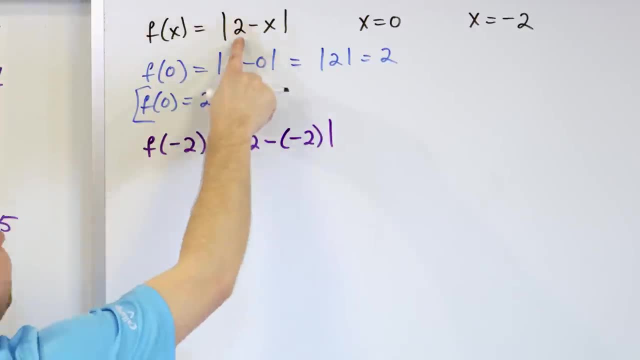 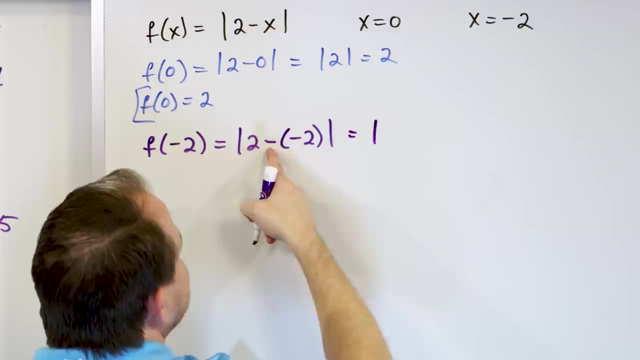 wrap it in parentheses Just to make sure you don't make any mistakes: 2 minus whatever x is, which is negative. So wrap it up like that And then you'll have 2, and this negative times negative gives you positive, which. 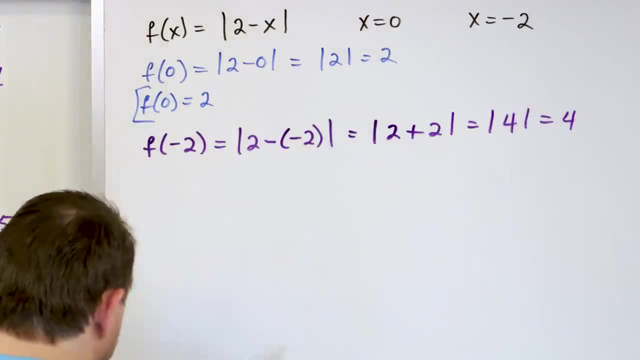 equals absolute value of 4,, which equals 4.. So you write your final answer as f of negative 2 is 4.. All right, So again we're not doing anything too crazy, We're just kind of getting practice with evaluating. 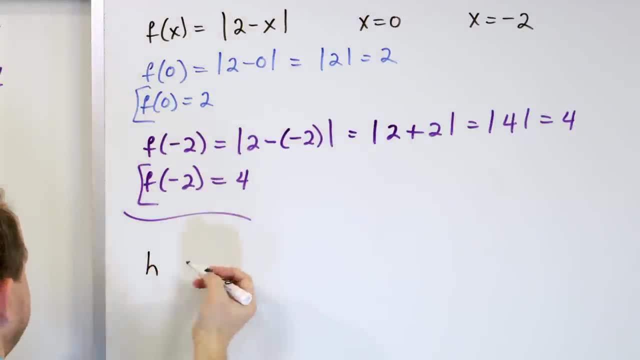 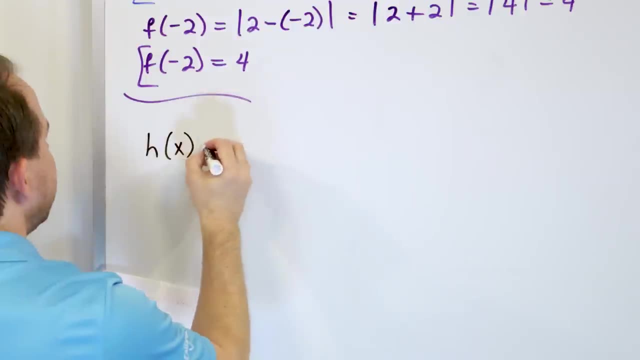 So what if you had the function h, which is pretty unusual to use h for a function name, but you can. You can use anything you want. h is a function of x and that's going to be equal to 10 divided by x squared plus 1.. 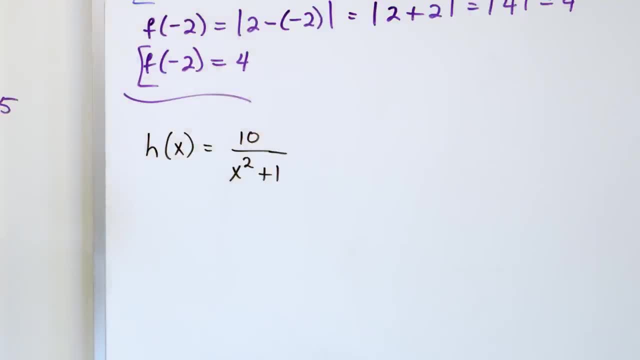 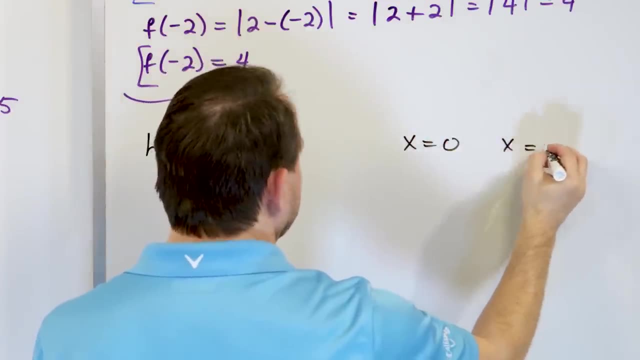 10 divided by x squared plus 1.. Complicated looking function right. You would definitely have to plot points to figure out what this is going to look like. Let's evaluate it: at x is equal to 0, and also at x is equal to 1.. 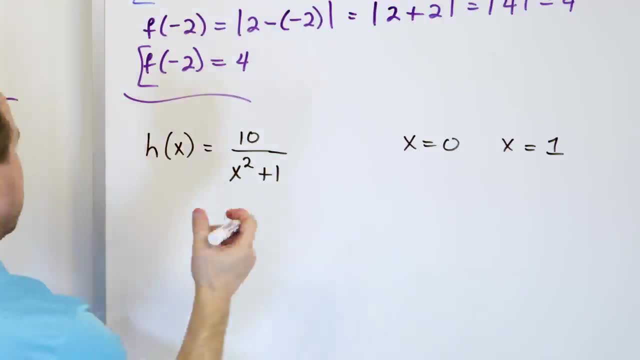 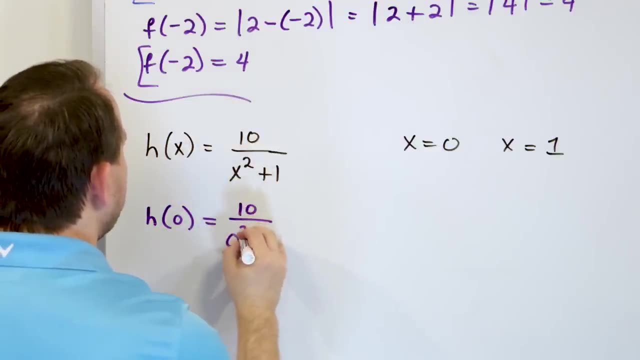 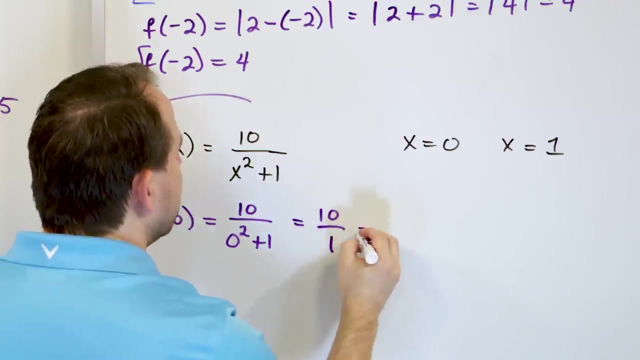 All right. So for the first one, We have h evaluated at 0.. Here we just plug the value in 10 over 0, squared plus 1 in the bottom. So what we have is 10 over. this is just going to be 0,. this is going to be 1, which means 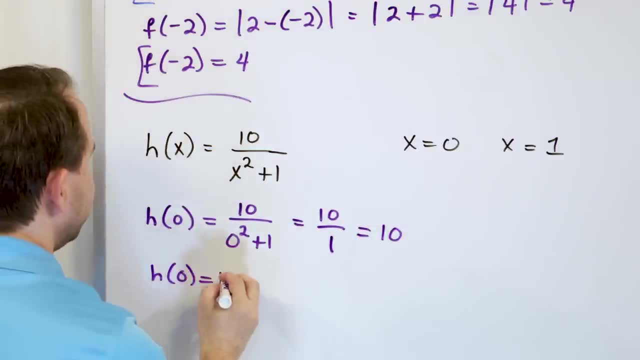 you're going to get 10 as the answer. So h evaluated at 0 is 10.. That's the final answer for this, And then we'll evaluate now. at x is equal to 1.. So h evaluated at 1 is 10.. 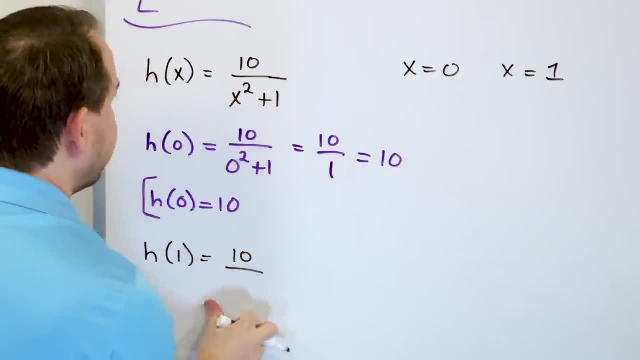 10 over x- whoops, not x. we're going to have to substitute in for 1 now 1 squared plus 1.. So we'll have 10 over. this is going to give you 1.. So 1 squared is 1.. 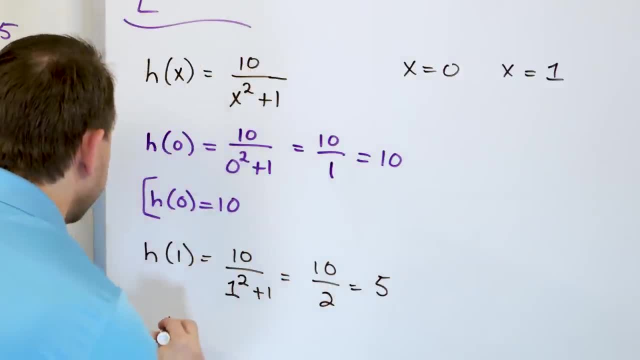 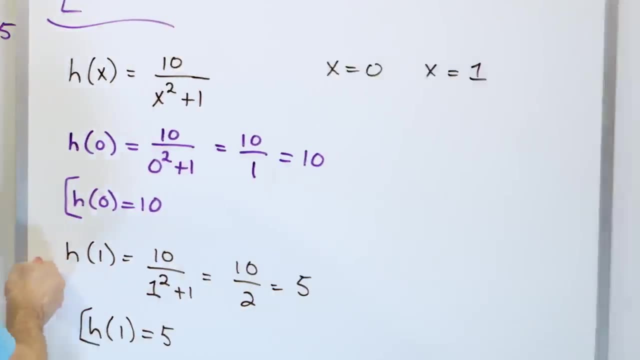 1 plus 1 is 2, which is going to give you 5.. So h, evaluated at 1, is 5.. All right, I only have one more, Just to give you a little practice. what if your function looked like getting a little? 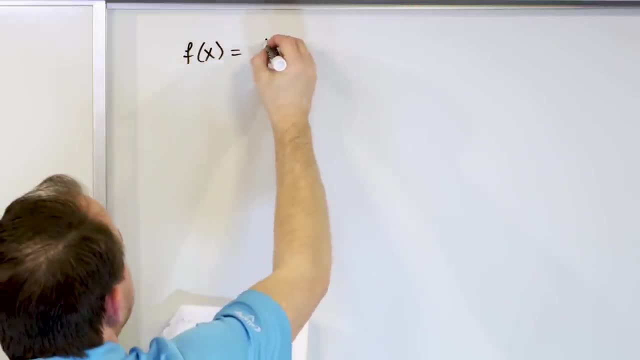 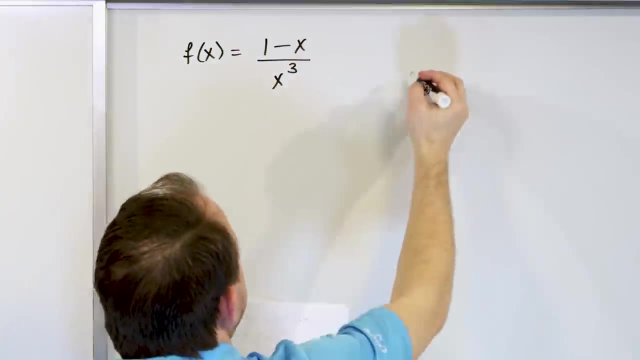 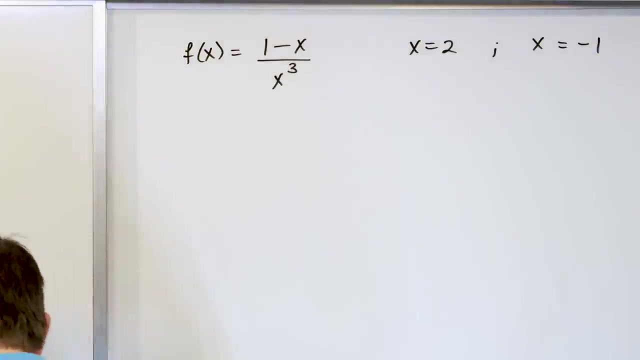 more complex now: f of x. f of x is equal to 1 minus x on the top divided by x cubed on the bottom. And we wanted to evaluate this at x is equal to 2.. And again we want to evaluate it at x is equal to negative 1.. 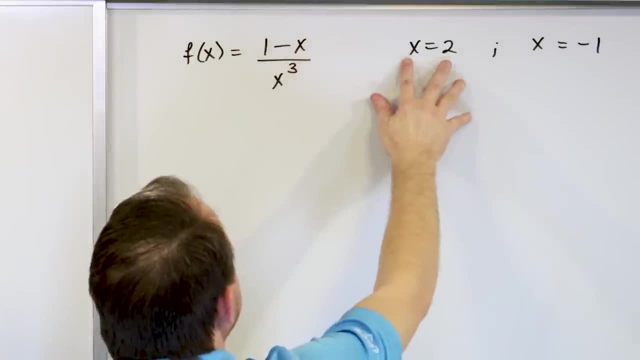 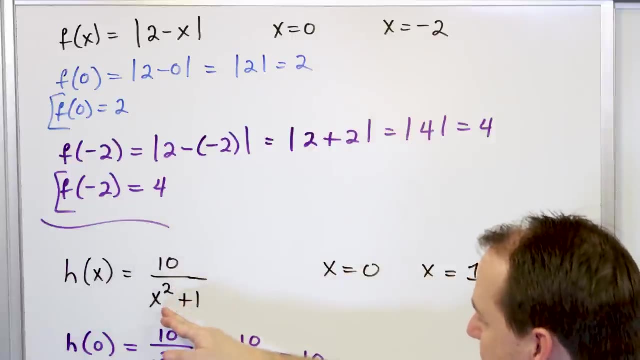 So again you have to go through the mechanics of the algebra, but basically it's the same thing. You stick the value of x in two locations. Notice, in all of these previous ones we had an x here, we had an x here and for the other. 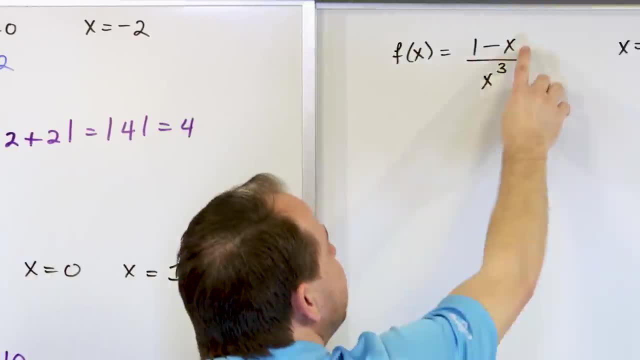 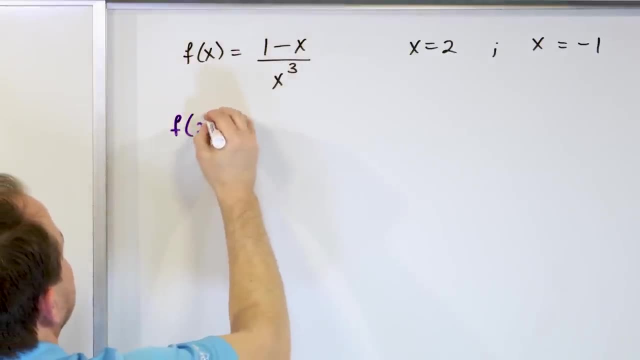 ones. we only have one value of x Here. We have an x value in two different locations, but it's the same thing. You just stick this value of x in both locations. So what we have is f evaluated at 2 is 1 minus 2 on the top, because we're sticking 2 in. 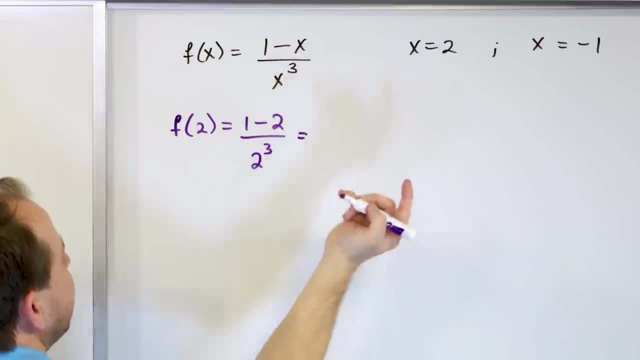 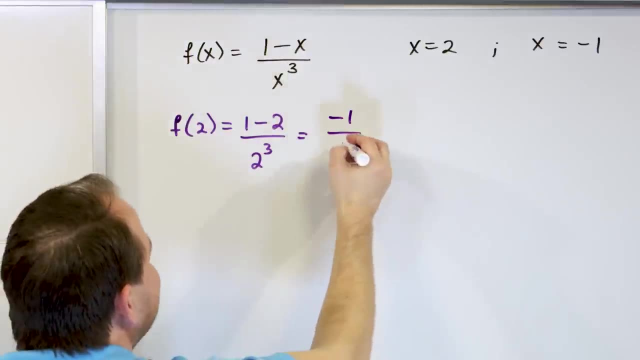 there, And then it's 2 cubed on the bottom. Now what is 1 minus 2? It's negative 1.. Now what is 2 cubed? That's 2 times 2 times 2.. So 2 times 2 is 4,, 4 times 2 is 8, so you have 8.. 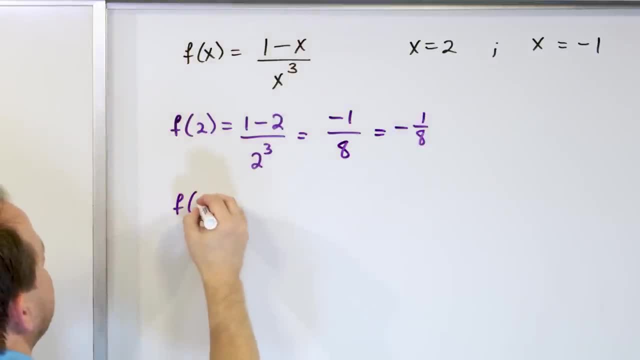 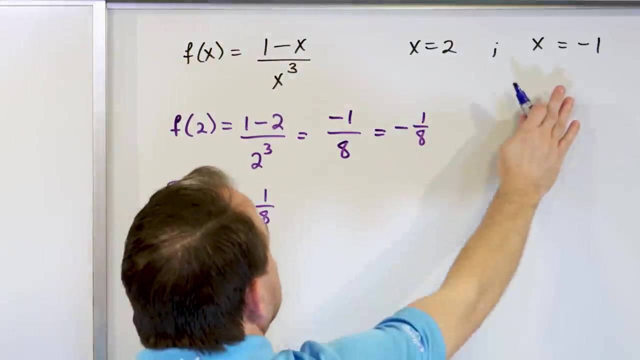 So what you have is negative 1 eighth. So you write it as: f, evaluated at 2, is negative 1 eighth, And it's perfectly fine to get fractions for answers when you're evaluating functions. Now for our last one, or I should say our next one. here we're going to evaluate at 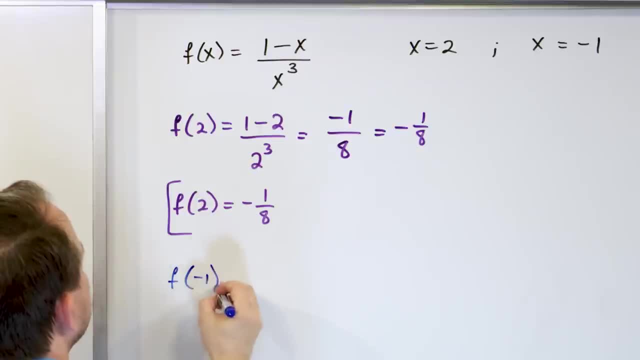 x is equal to negative 1.. You say f, evaluated at negative 1 is 1 minus. now here you have to be careful: 1 minus, but x is negative. So you should wrap it in parentheses to make sure you don't make any mistakes. 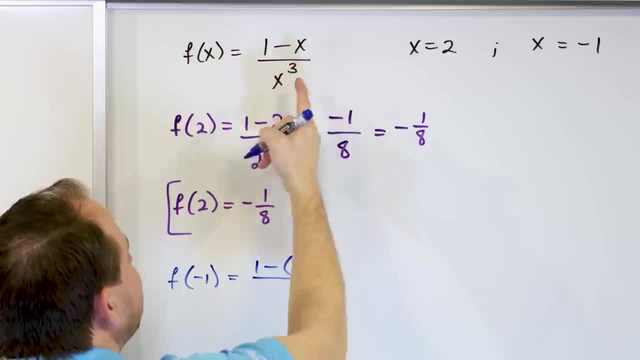 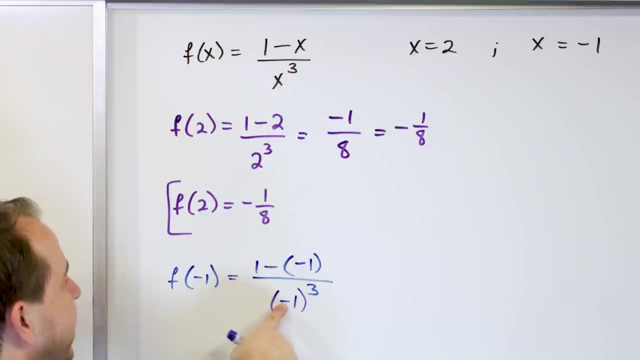 1 minus this value of negative 1.. And same thing. on the bottom It's negative 1 cubed. You should wrap it in parentheses to make sure you don't make any sign errors, Because if you don't put the parentheses here you might forget to cube the negative sign. 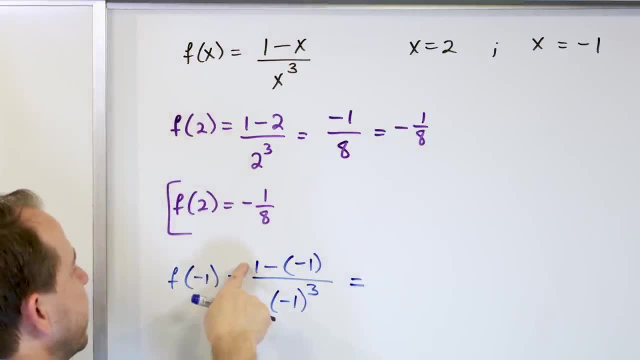 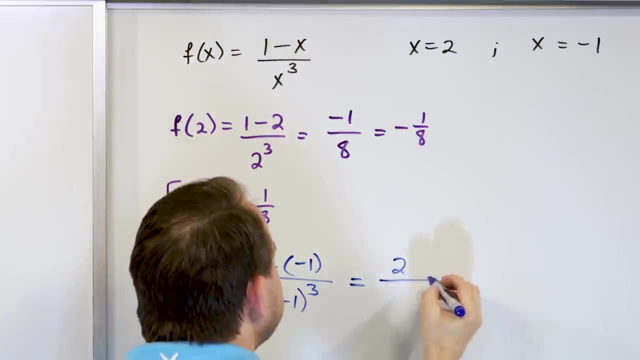 as well. Now, on the top, what you have is you have the 1 minus negative 1, so you have double negatives here, so it becomes a plus, So it's 2.. And on the bottom, I'm going to help you out and write it like this: 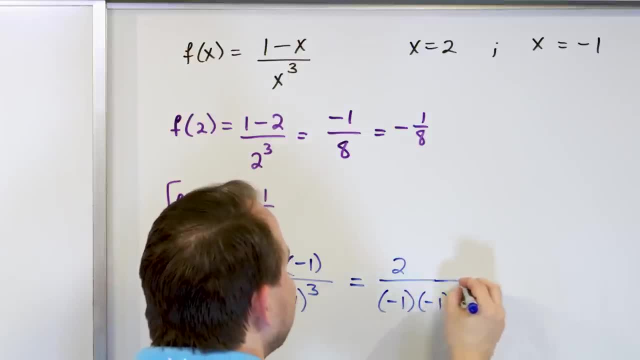 This is negative, 1 times negative, 1 times negative, 1.. That's why I say it's important to wrap the parentheses to make sure you carry the signs through. So here now you can see that you have on the top you have 2, but on the bottom you 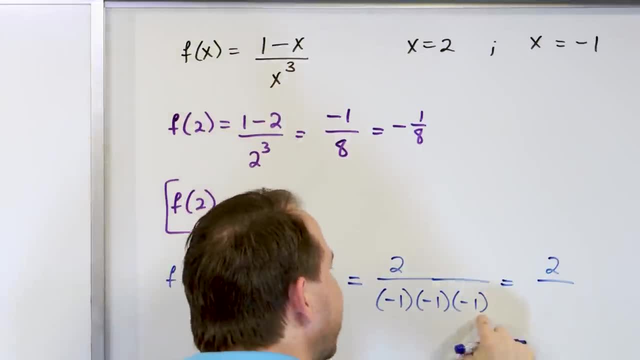 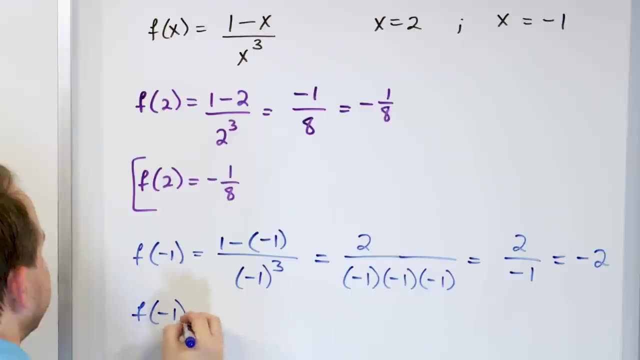 have negative 1. times negative 1 is positive 1, but times another negative 1 gives you negative 1.. So the answer you get is actually negative 2 for the answer And this function, evaluated at negative 1, is negative 2.. 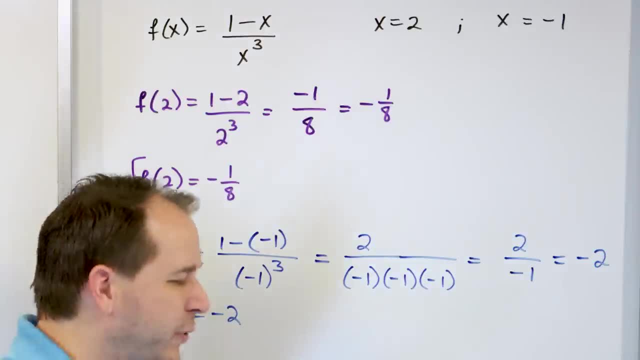 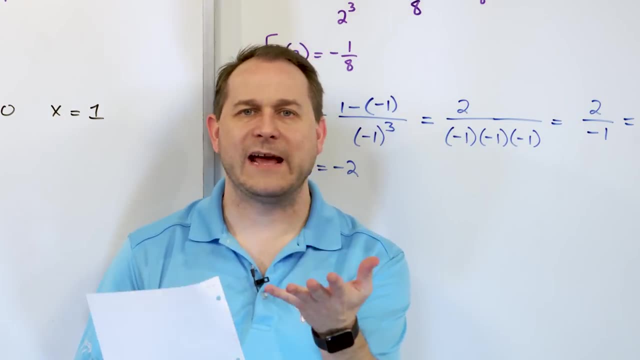 And that's the final answer. So in this lesson we wanted to re-emphasize the idea of a function Being a machine that takes a mathematical machine that takes input values, performs a calculation. Whatever the function happens to be, that's the calculation that's done. 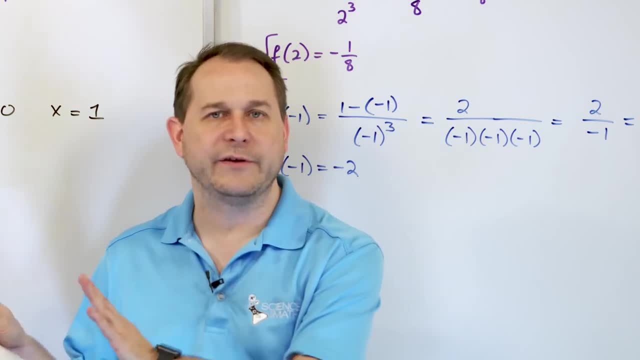 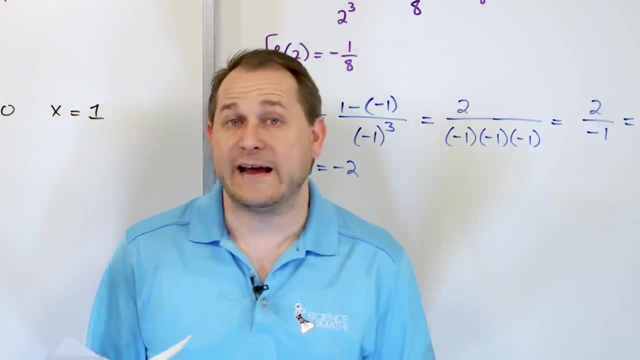 And then you get outputs that we call f. So here we just started with very simple functions, working our way through the complexity, mostly getting practice with substituting in and doing the algebra. But this is how functions are evaluated. Now we have another lesson here. 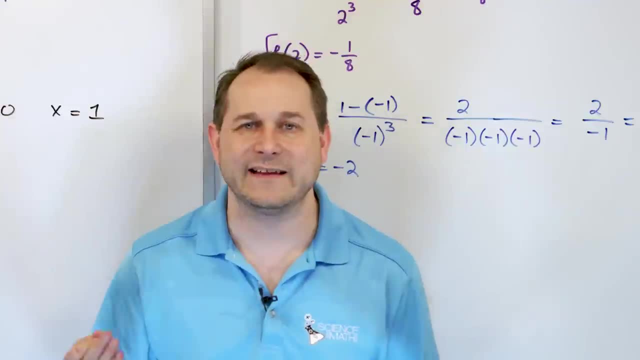 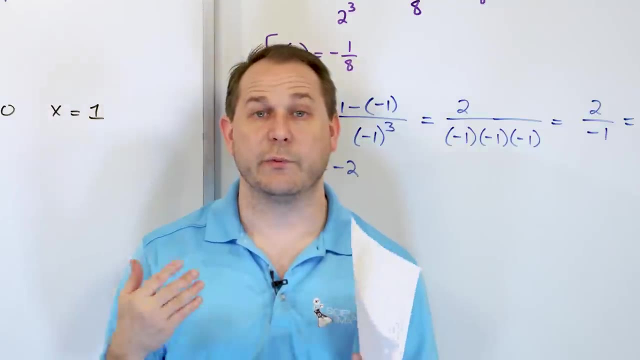 We're going to have slightly more complex functions, but in the next lesson we'll have exactly the same concept of plugging this guy in and evaluating. So make sure you can do all of these problems and then follow me on to the next lesson, where